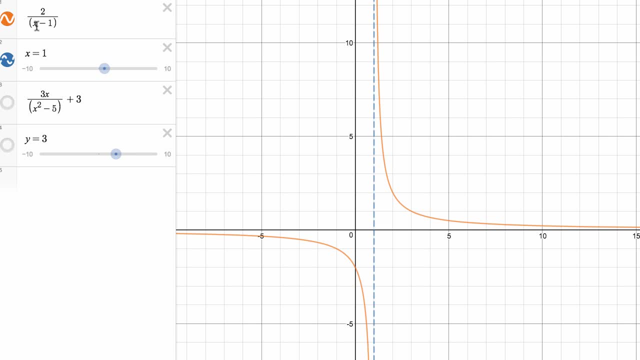 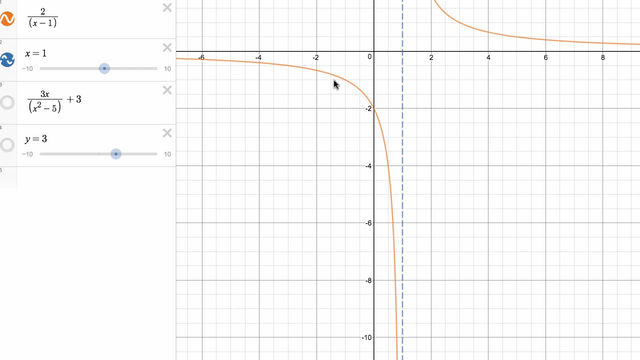 of f of x is equal to two over x minus one, And we could think about it from the left and from the left. So if we approach one from the left, let me zoom in a little bit over here So we can see as we approach from the left. 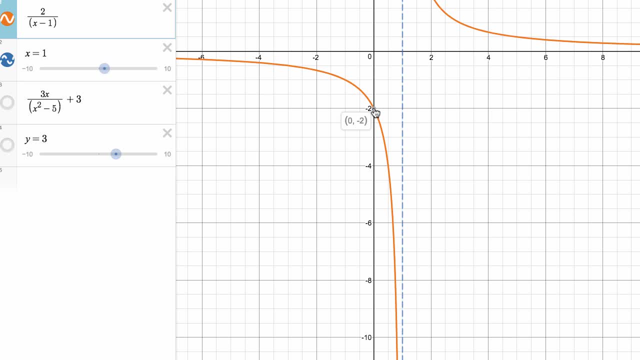 when x is equal to zero, the f of x would be equal to negative two. When x is equal to 0.5, f of x is equal to negative four. And then it just gets more and more negative the closer we get to one from the left. 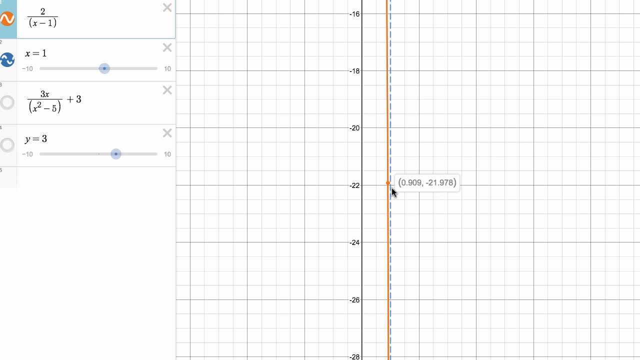 I could really, so I'm not even that close yet. If I get to, let's say, 0.9, 0.91,, I'm still nine hundredths less than one. I'm at negative 22.222 already. 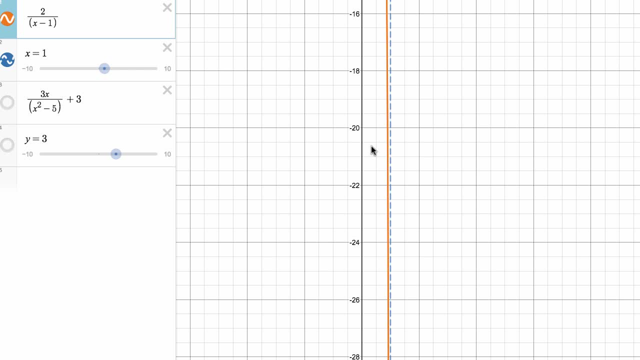 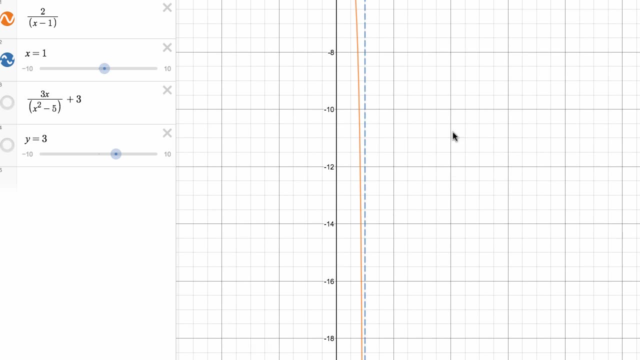 And so the limit as we approach one from the left is unbounded. Some people would say it goes to negative infinity, but it's really an undefined limit. It is unbounded in the negative direction, And likewise as we approach from the right, 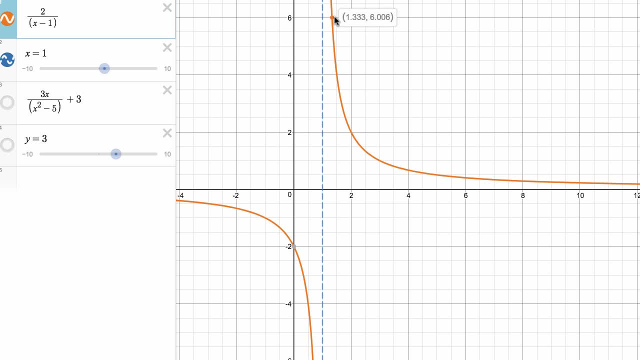 we get unbounded in the positive infinity direction And technically we would say that that limit does not exist. And this would be the case when we're dealing with a vertical asymptote like we see over here. Now let's compare that to a horizontal asymptote. 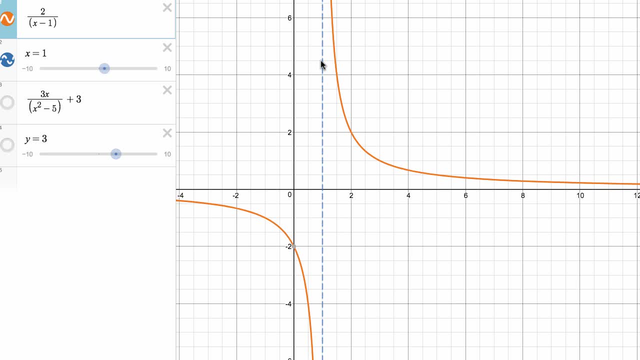 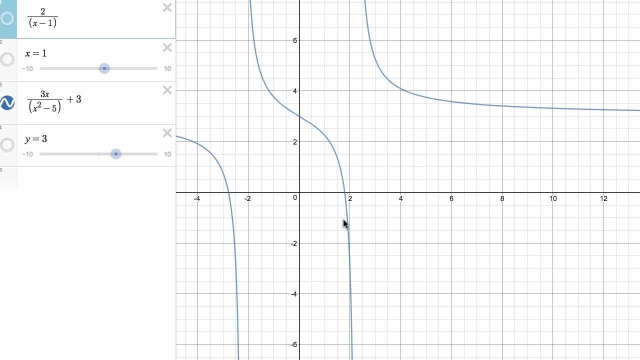 where it turns out that the limit actually can exist. So let me delete these, or just erase them for now. And so let's look at this function, which is a pretty neat function. I made it up right before this video started, but it's kind of cool looking. 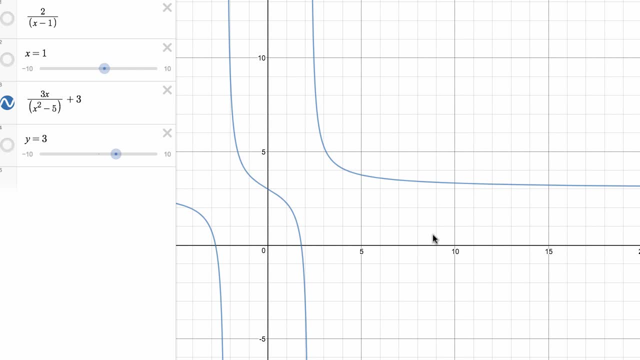 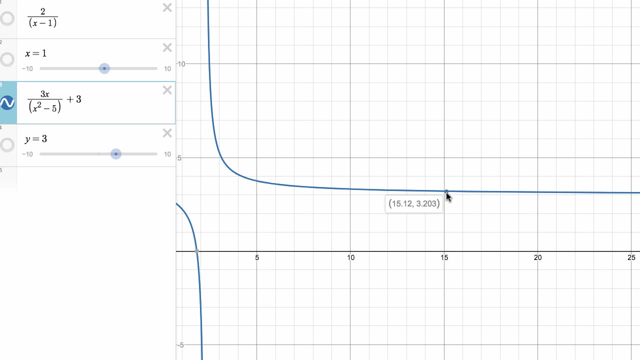 But let's think about the behavior as x approaches infinity. So as x approaches infinity, it looks like our y value, or the value of the expression, if we said y is equal to that expression. it looks like it's getting closer and closer. 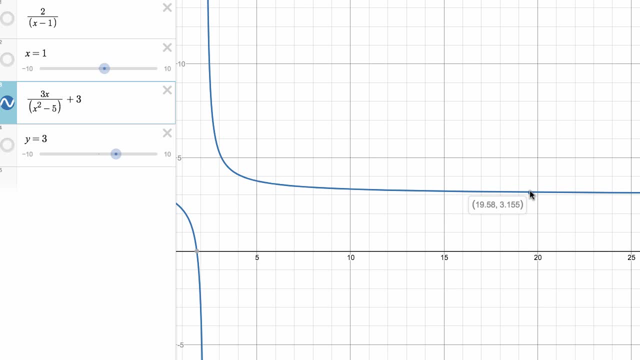 and closer to three, And so we could say that we have a horizontal asymptote at y is equal to three. And we could also- and there's a more rigorous way of defining it- say that our limit, as x approaches infinity, is equal of the expression or of the function. 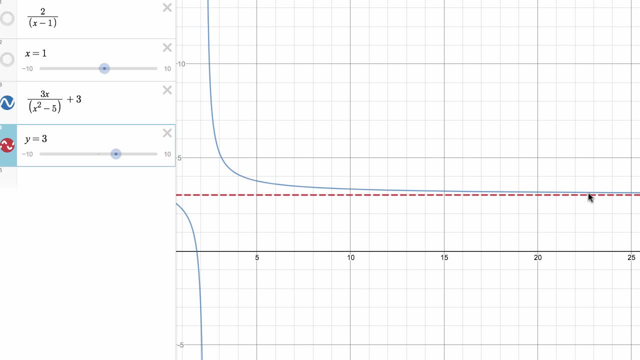 is equal to three. Notice my The mouse is covering it a little bit. As we get larger and larger, we're getting closer and closer to three. In fact, we're getting so close now that, well, here you can see it.